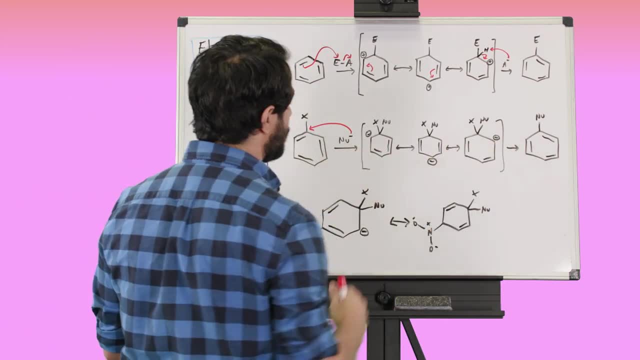 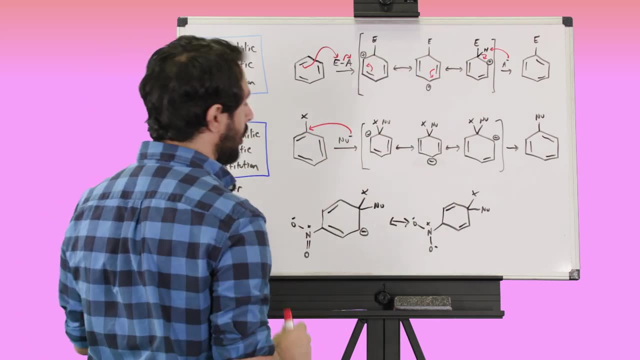 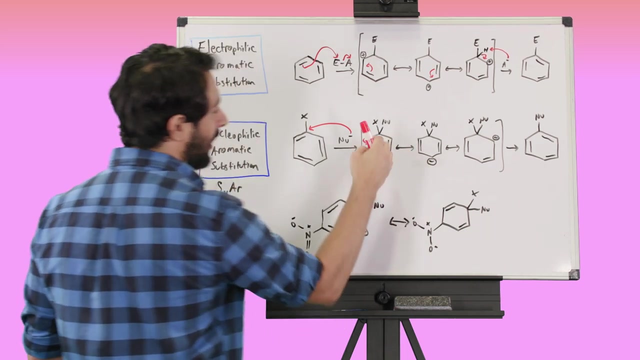 positive site on the molecule, and now we've got again some intermediates here, but now notice that each of these resonance structures has a negative charge on there instead of a positive charge like with EAS. So again we've got some resonance, so this can move over here. right, we can get this. 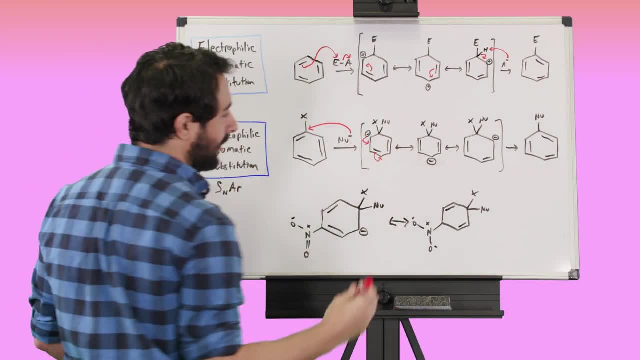 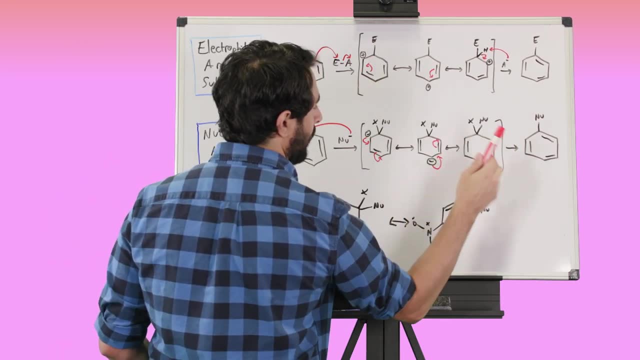 negative charge down there and that will pop this pi bond up there to give us this one, and then again we can move this right here, which will pop this bond over there, put the negative charge over there. So these are the intermediates and then so, as you would expect, again we're gonna. 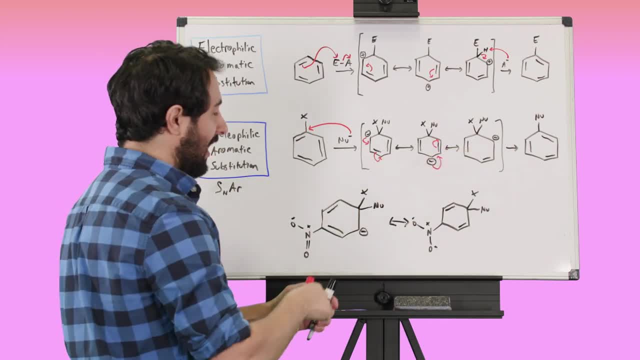 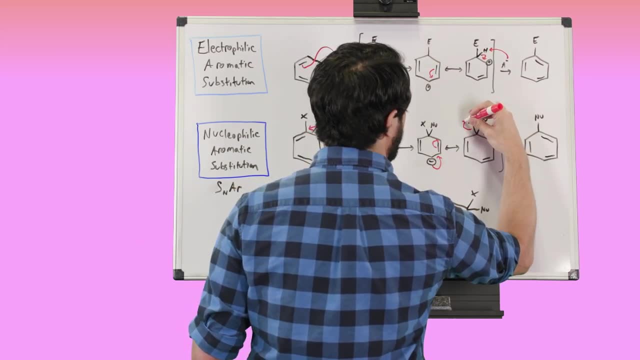 expect again. that is the slow step. the generation of this intermediate is the energetically unfavorable step, and then this can go ahead and kick this off. We're gonna kick off the leaving group, So that is gonna leave some other nucleophile. so this is a group that would have been difficult. 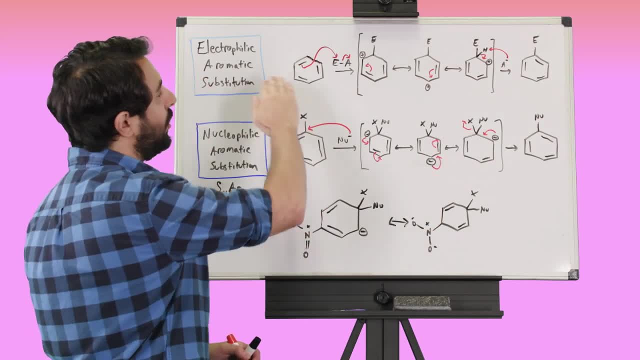 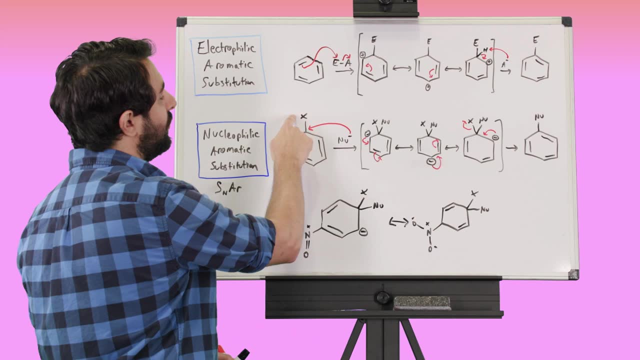 to get onto a benzene ring. initially because, right, we're used to putting electrophiles on benzene, so now we're figuring out a way to put nucleophiles on there as well. But we were able to do it because of this halogen there. 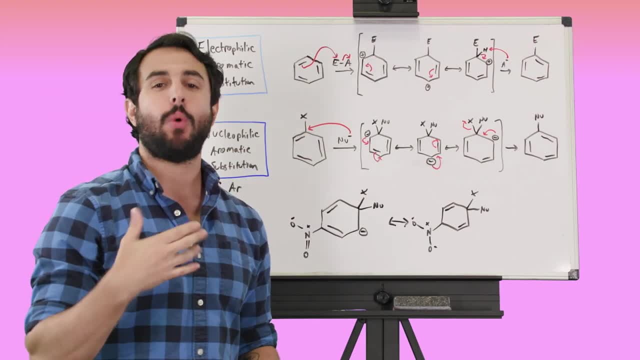 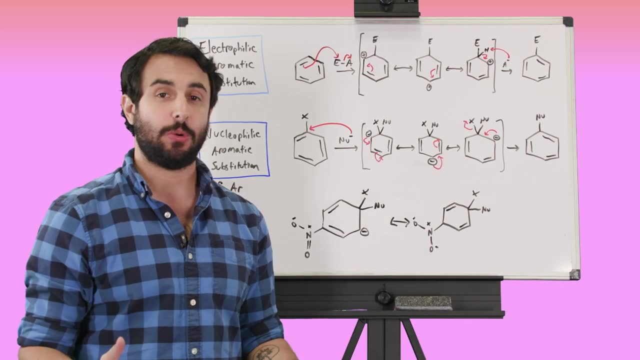 So this is a topology, This is a type of nucleophilic substitution, but it's quite a bit different than any other type of nucleophilic substitution that we've seen. So remember, if we go back, we know about SN2, but with SN2, as well as SN1, we're dealing. 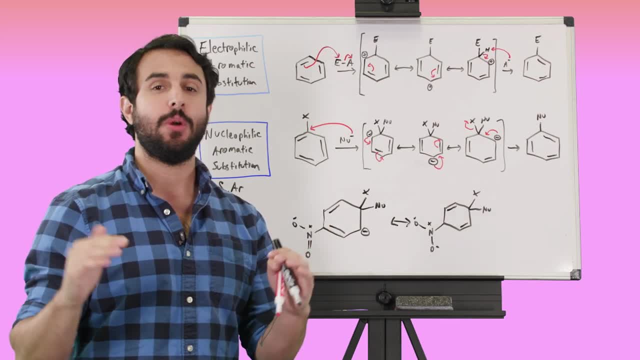 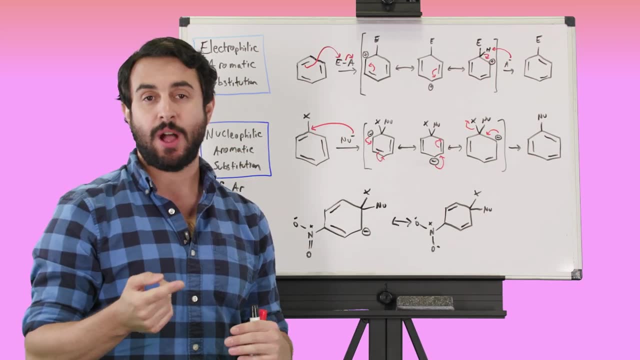 with SP3 centers. So for SN2, we've got the nucleophile coming in and the leaving group leaving all at the same time. That's a concerted reaction. Then with SN1, we saw a leaving group leave and then we had an intermediate, and then 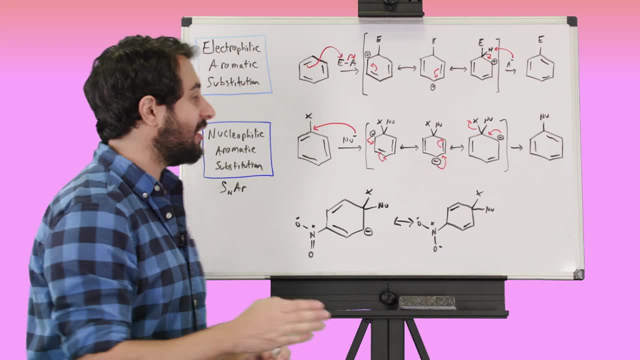 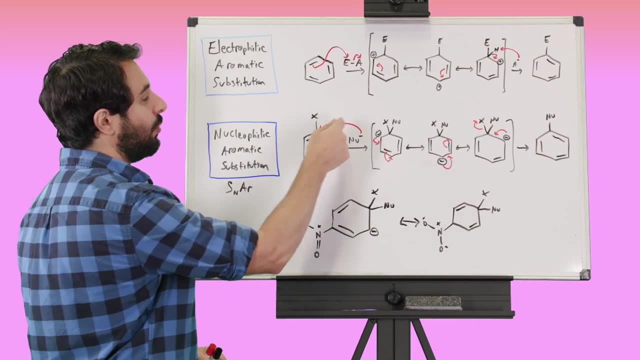 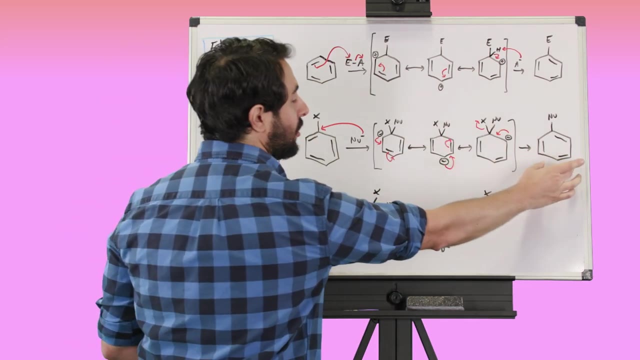 in a separate step, the nucleophile attacks. Well, now we have a different situation, where a nucleophile is attacking an SP2 center and now it is the reverse situation, where we have a nucleophile attacking, then we have an intermediate and then, in a second step, the leaving group leaves. 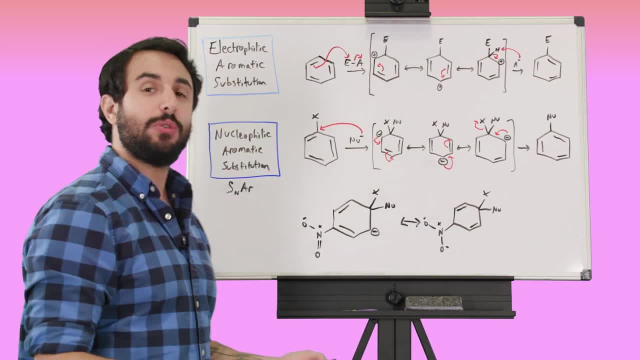 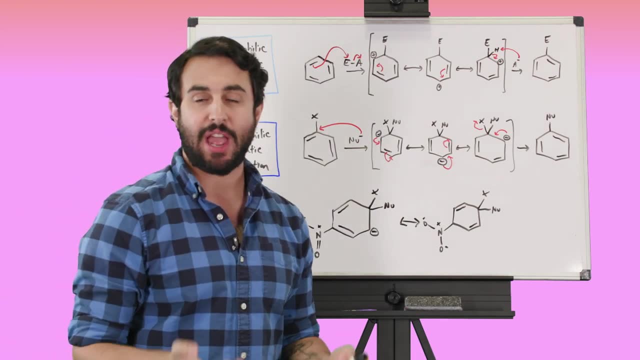 So that leaves us this here, and so this is a completely new type of nucleophilic substitution, which is abbreviated this way: SNR. So the thing that it has in common with electrophilic substitution is that the first step is the 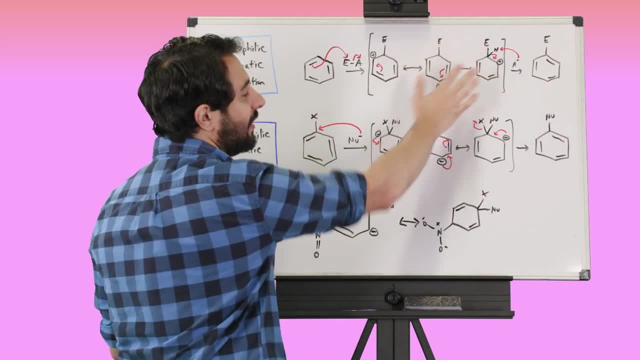 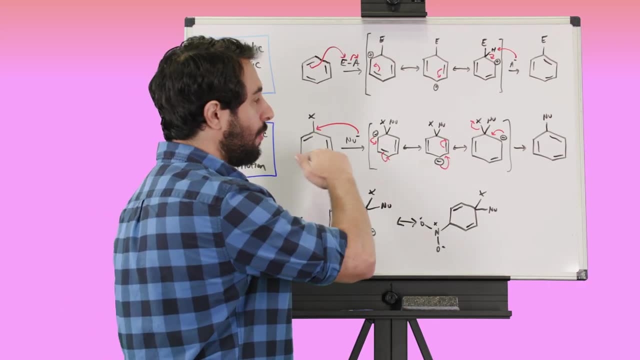 slow step. We've got a stable molecule and then we're generating a relatively unstable intermediate. So we need to understand some ways that we can promote this first reaction. If we want to do this reaction, we want to make it a little more energetically favorable. 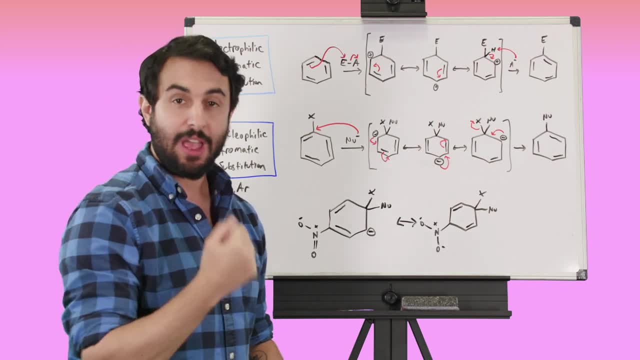 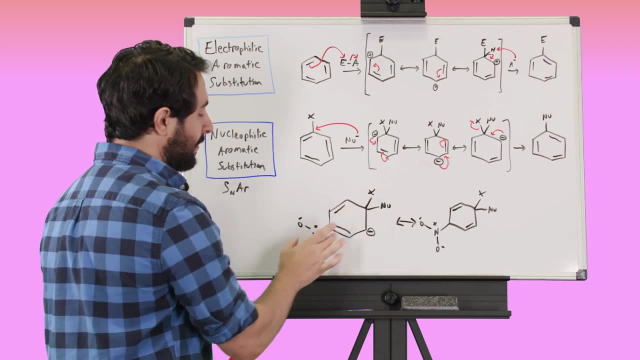 and the way we do that is by putting electron withdrawing groups on the benzene ring. So let's say we're trying to do some nucleophilic aromatic substitution and on this molecule there was a nitro group. so we know that nitro groups are electron withdrawing by resonance. 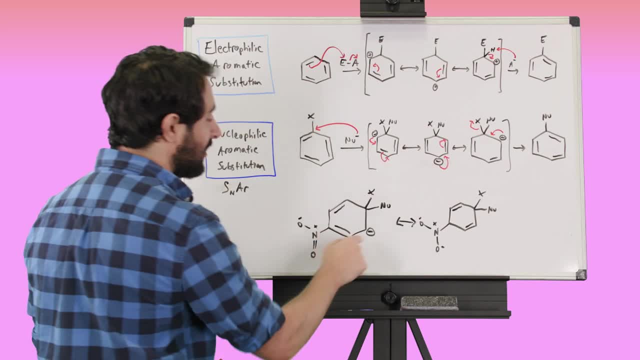 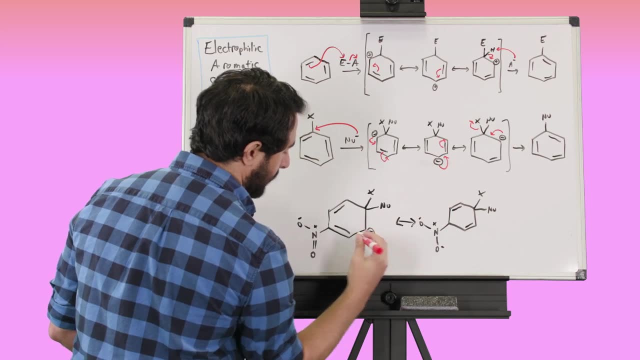 because of the positive charge on that nitrogen. So let's say this is our intermediate. What we want to notice that's interesting about the resonance here is that we can do this, We can push this over here, and then we can push this all the way up to that oxygen there. 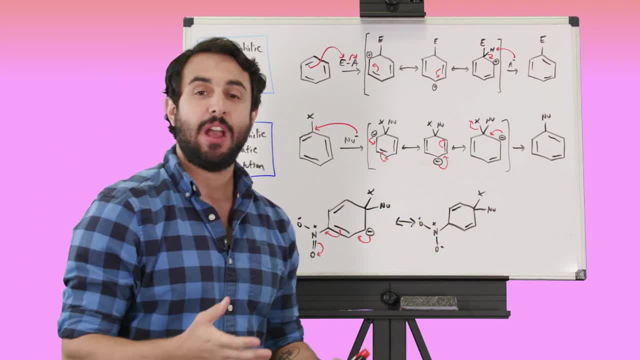 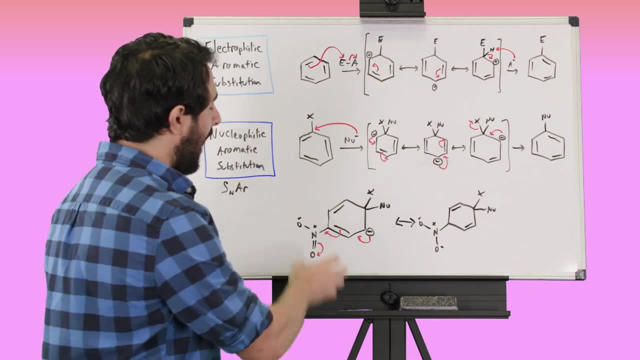 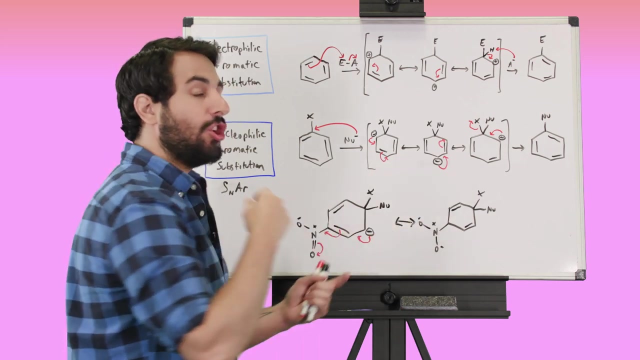 So that's going to give us this intermediate. So we know that any time we distribute electron density along a greater portion of the molecule, that's a stabilizing effect, and so that's why having electron withdrawing groups on the molecule is going to stabilize that intermediate, just the same way that electron donating. 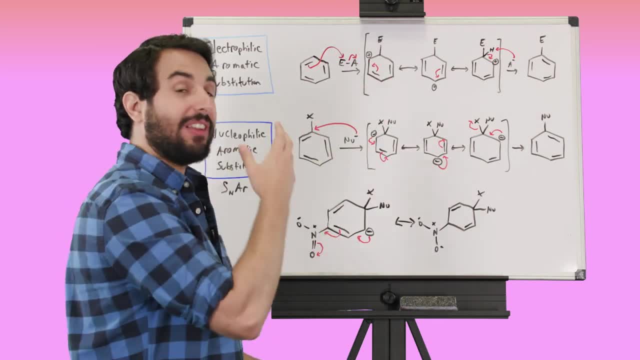 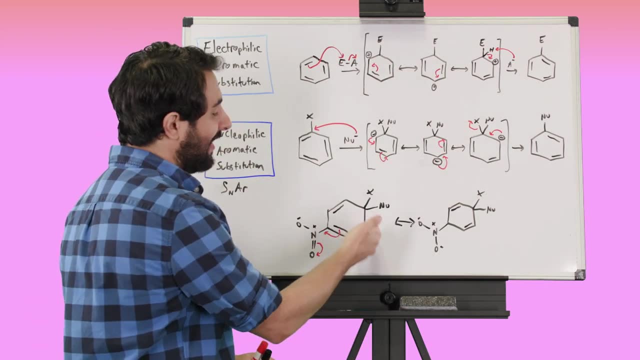 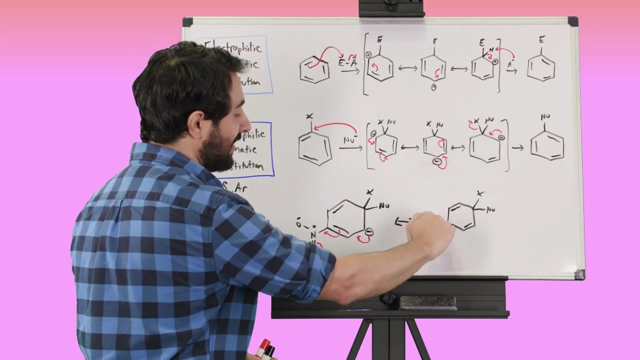 groups were able to stabilize the intermediate for electrophilic aromatic substitution because we had a positively charged intermediate so more electron density was stabilizing that. Here we've got a negatively charged intermediate, so anything that withdraws some of that negative charge into some substituent is going to stabilize that intermediate. 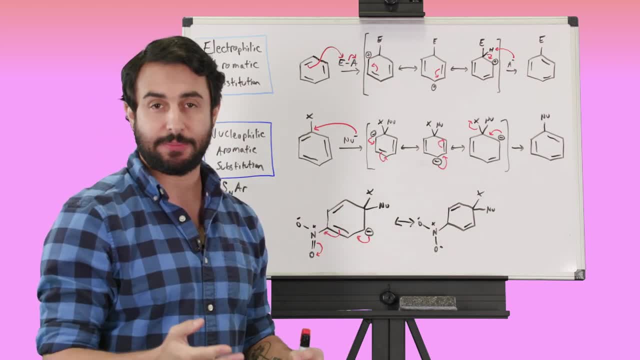 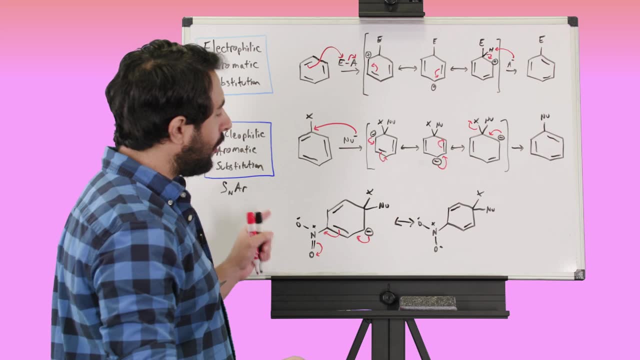 So, typically, when we are going to be doing nucleophilic aromatic substitution, you're going to see nitro groups, Nitro groups and some other electron withdrawing groups on those molecules in order to get them to go. and we know that this is true because if we put several nitro groups, if 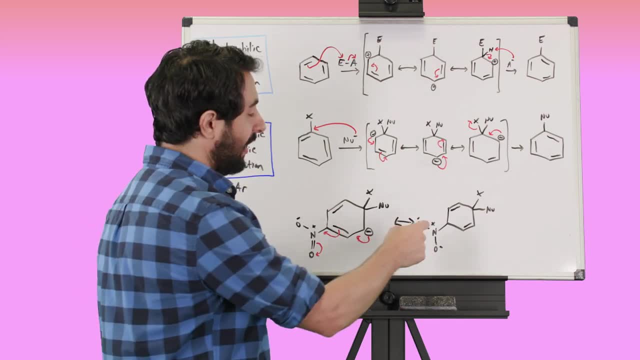 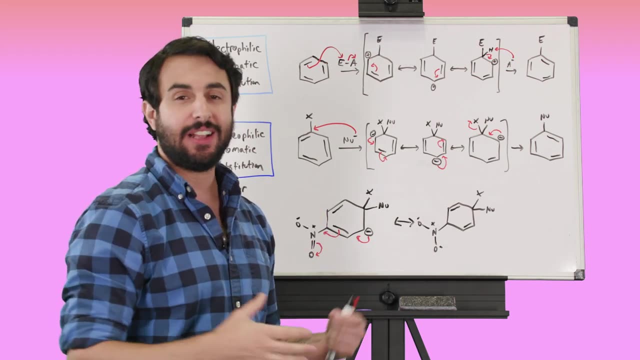 we put, say, three nitro groups on there, we can actually isolate that intermediate. It's called a Meisenheimer adduct, So we're able to crystallize that and isolate it, and so that is very firm empirical evidence of this mechanism. 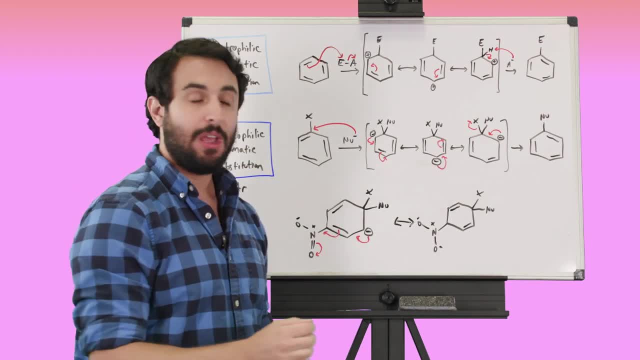 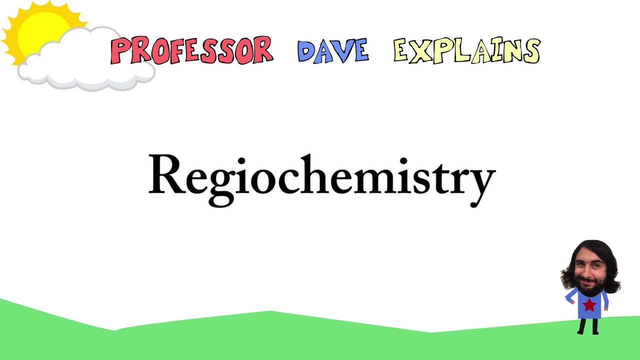 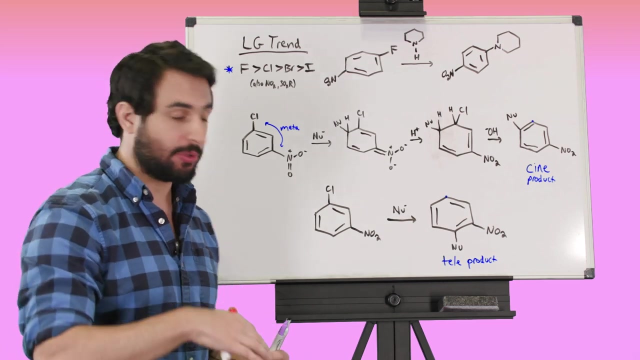 So now that we understand the basics about the mechanism for nucleophilic aromatic substitution, let's go ahead and take a look at some examples. So, in order to do nucleophilic aromatic substitution, we know that we need to have a leaving group on the substrate, and so we want to notice something that's a little bit interesting. 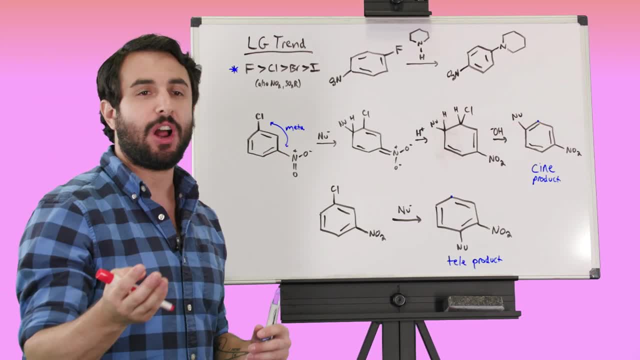 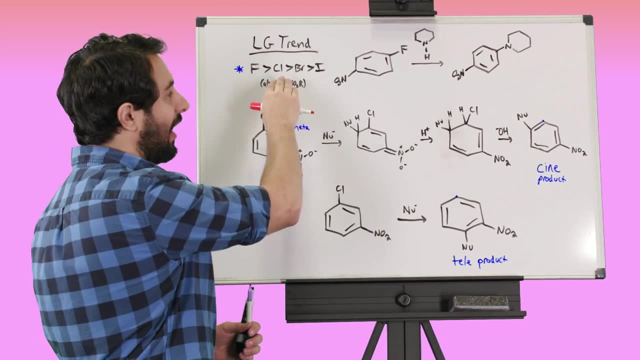 about leaving group trend. Usually when we're looking at other situations where we see leaving groups- if we're looking at the halide ions, usually it's the iodo group is the best leaving group and then it gets worse as they get smaller because they're less stable. 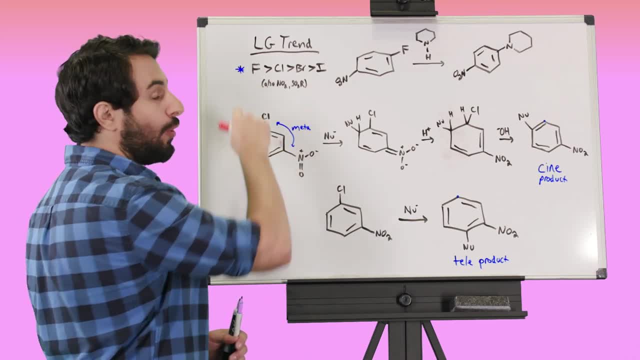 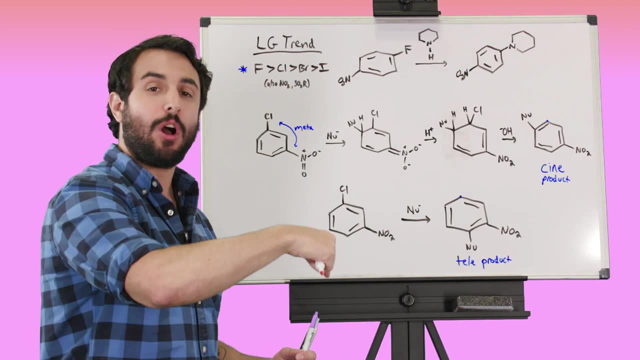 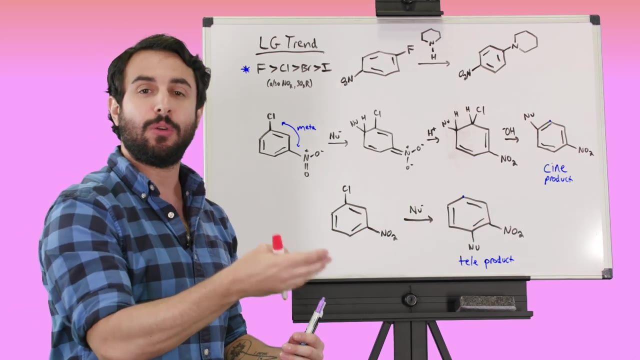 But for this it's not, It's actually different. We see that the fluoro group is the best leaving group in this context, and the reason is that the nucleophile has to attack the carbon where the leaving group is, And so the more polarized that bond is, the more readily it will attack that carbon, because 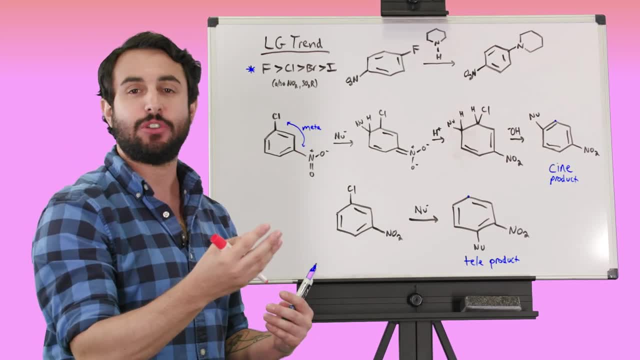 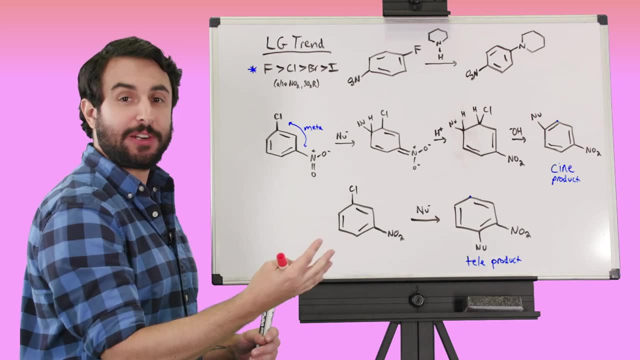 that's the slow step. So anything that maximizes the energetic favorability of the nucleophile attacking that carbon is going to help the reaction go. And so because fluorine is the most electric Electronegative, that's the most polarized carbon-halogen bond, and so fluorine is actually 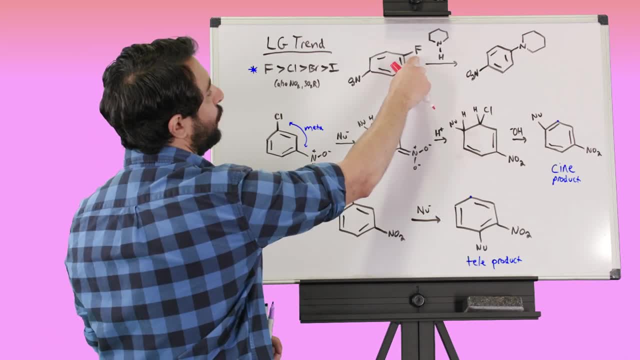 going to be the best to get these to go. So here's an example: We see a fluoro group on there, para-2,, this nitro group, and then we're going to do nucleophilic aromatic substitution with this amine. 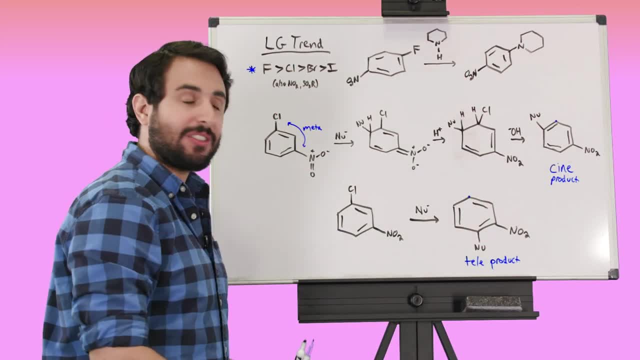 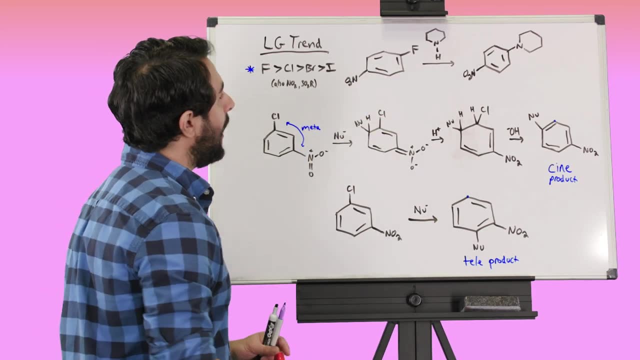 So we're going to go ahead and pop the amine on there and that's how we get that product. So this is a classic example. We can get amines on there in this way, and so that's a pretty common example. 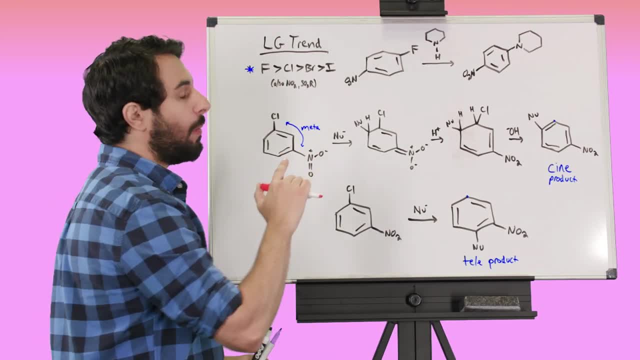 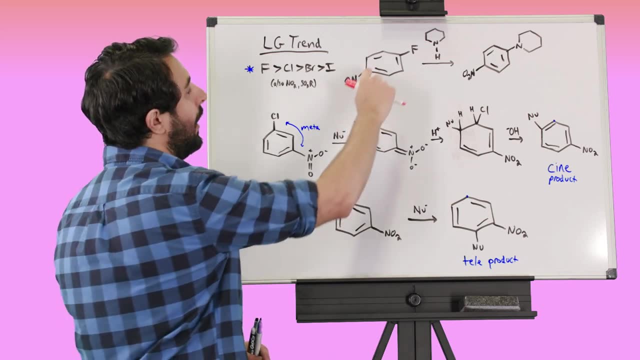 Now let's talk about one other aspect of regio Regio chemistry, because what we've looked at so far is we've had the electron withdrawing group that's helping the reaction go in a situation where it's para to the leaving group, and this will also work just as well if it's ortho. 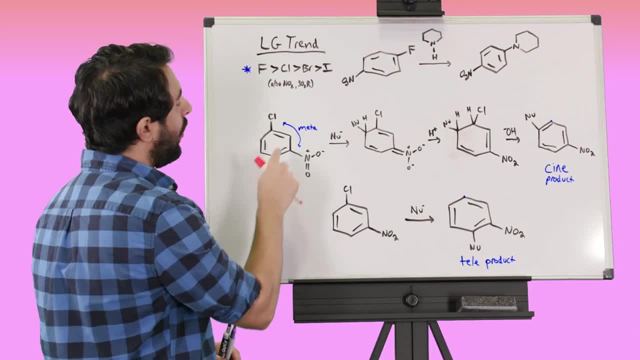 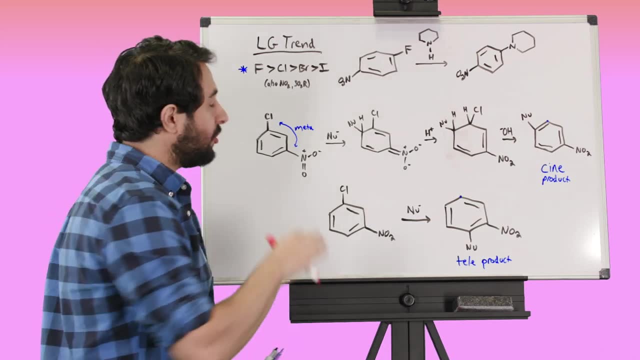 So ortho or para, that works well for the resonance. but what if we have a situation where the leaving group and the electron withdrawing group, like a nitro group, are meta to one another? So this is a little bit different, because let's say we have a nucleophile that's trying to 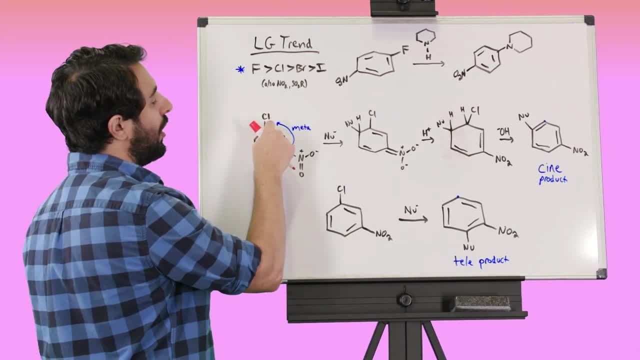 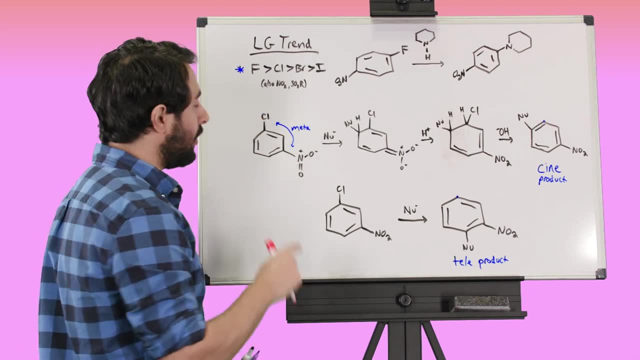 attack. Now it's not so clear where it's going to go. It's true that this is the most partially positive carbon. that is what we might expect in terms of where the nucleophile is going to go, but the resonance won't work out. 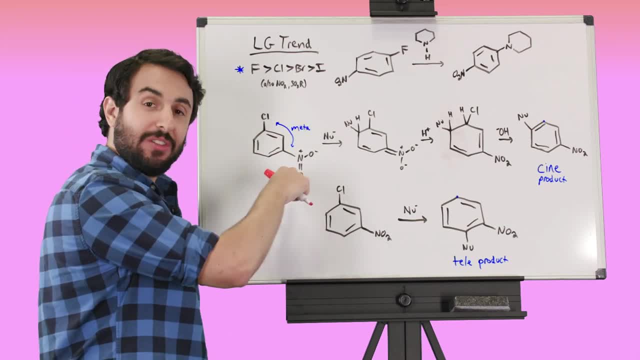 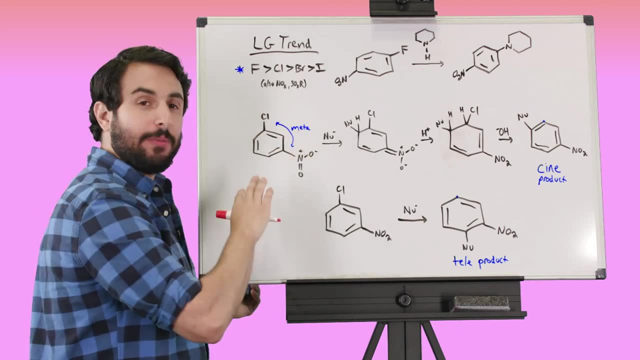 If it attacks there, the resonance can't get over to get pushed up into this nitro group, which is the feature that stabilizes the intermediate in the first place. So actually it's true that in often cases nothing is going to happen. it's just not. 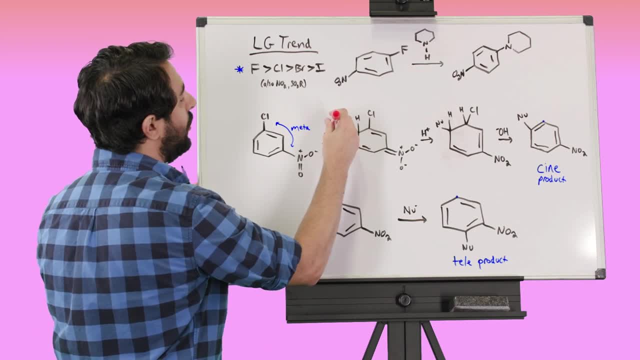 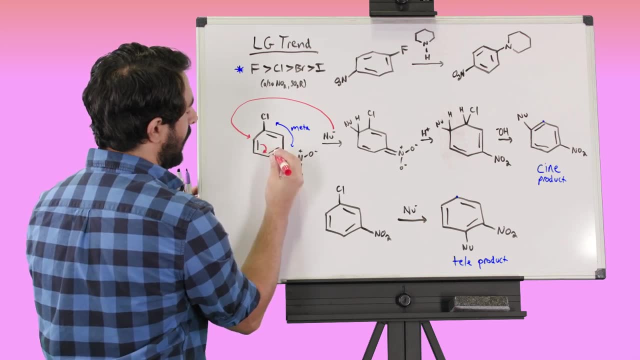 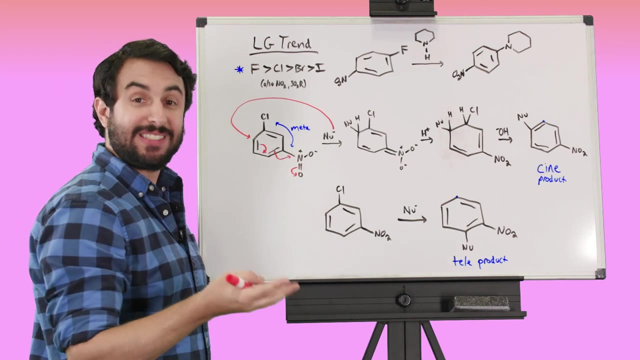 going to work out. But there are situations where it will attack. It will attack some other location. So let's say it attacks here and that way we can push these pi electrons all the way up into that nitro group. So remember, if we attack there, the polarization of that bond is a factor, but this is a bigger. 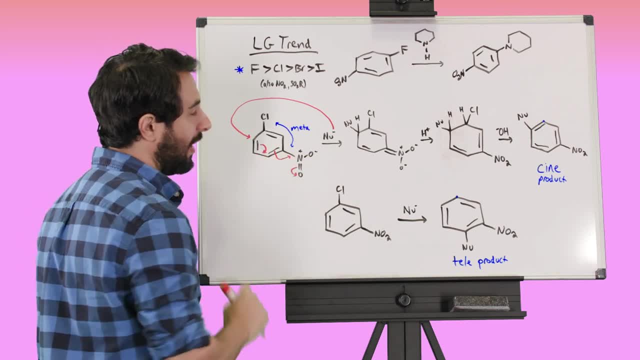 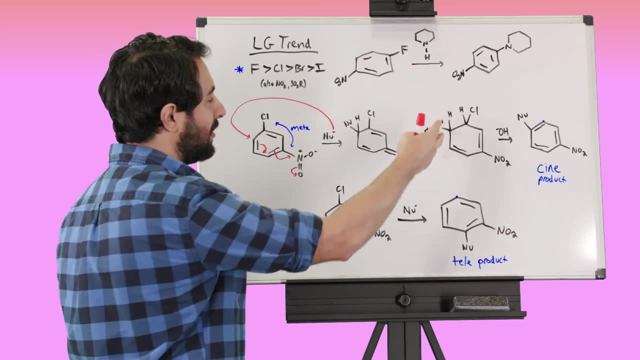 factor, where we want to be able to push the electrons by resonance all the way up to the nitro group. So we have this intermediate here. Now this is actually quite basic, so we could protonate from solvent. it could grab a proton of whatever solvent is in there. 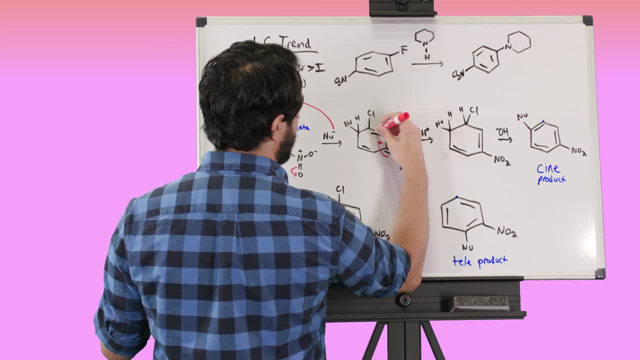 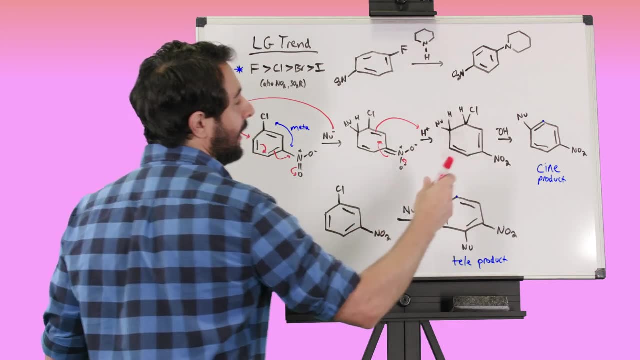 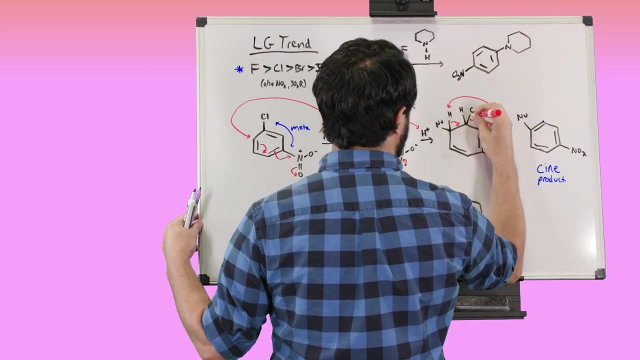 So let's go ahead and protonate that. We'll push this all the way up here and we'll protonate there And then the conjugate base of whatever offered that proton can go ahead and eliminate HCl. So let's grab that and let's put that there and let's kick off the chlorine. 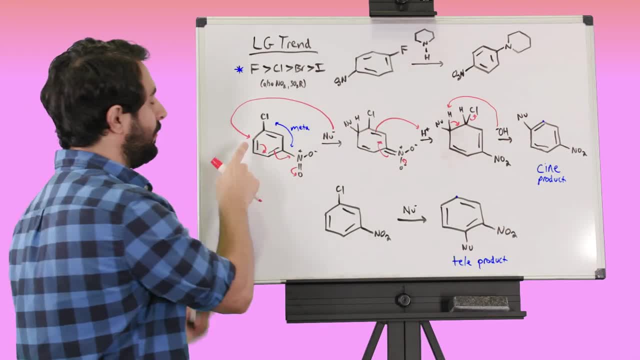 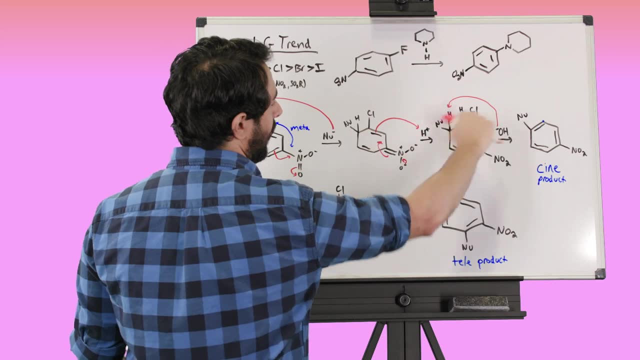 Okay, so all we've done is we had the nucleophile attack, but we had the nucleophile attack here in a different position, one away from the chlorine, and so then we just protonated and then did our elimination. So here is our product, but this is called the Sine product. 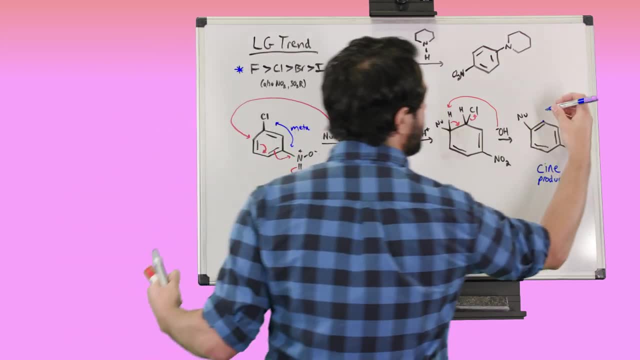 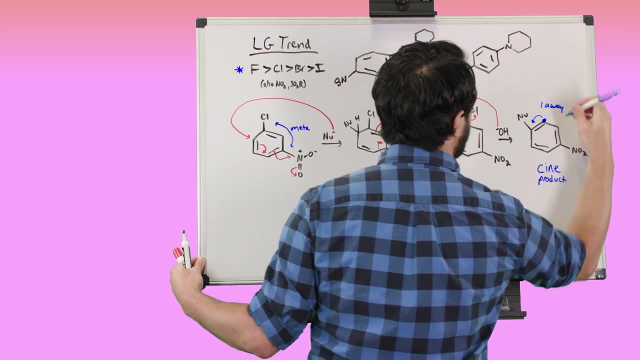 So we just did Sine substitution and we call it that because the nucleophile, the incoming nucleophile, is one away. right, We say it's one away from where the leaving group initially was. So we had the leaving group there, but the nucleophile came in there. 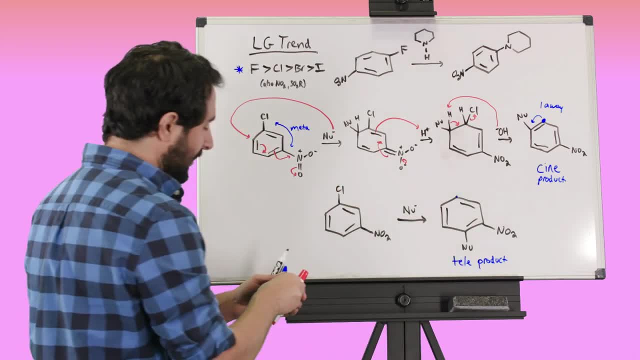 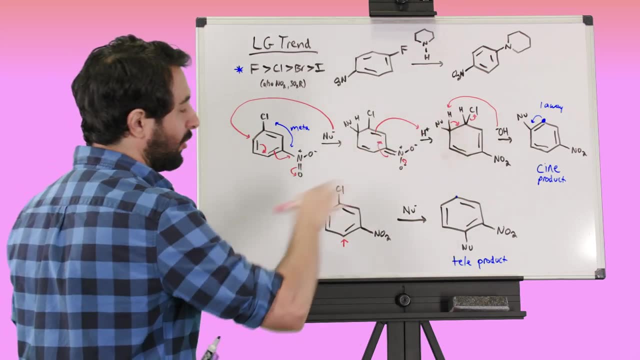 So that's the Sine product. okay. Now we can also see something else. We can see the nucleophile attacking here. Okay, So the mechanism is essentially the same. so I won't draw it all again. But if we do that, we get the Tele product. 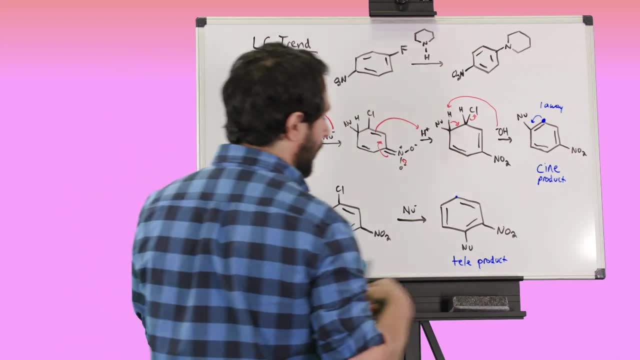 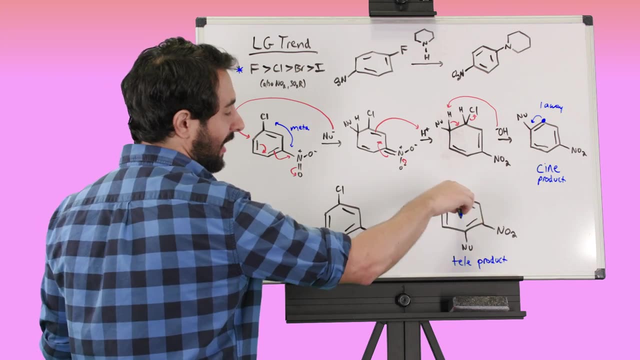 So this is Tele substitution and it's the Tele product, because the leaving group was here and now the incoming nucleophile is Para. with respect to that, It's on the opposite side of the ring. So this is the spatial orientation, or the regiochemistry that produces the Tele product. 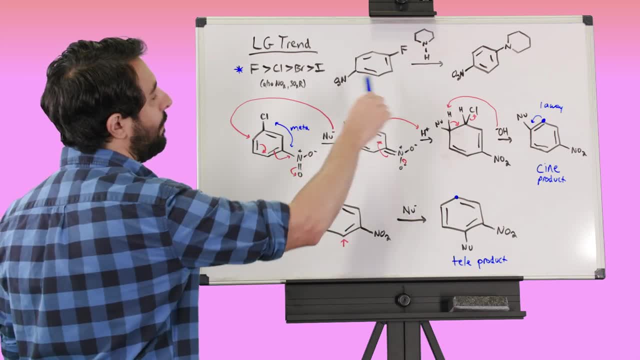 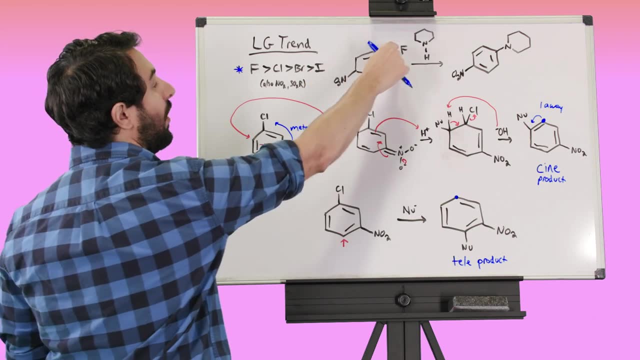 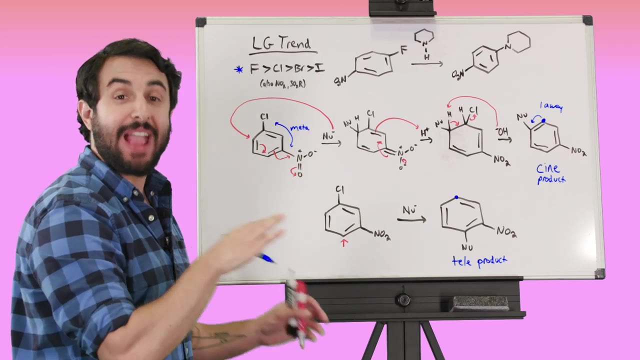 or Tele substitution. So now we understand a little bit more about the differing regiochemistry. Okay, So the difference between the two is that the electron withdrawing group is with respect to the leaving group and the sites where the incoming nucleophile will attack, depending. 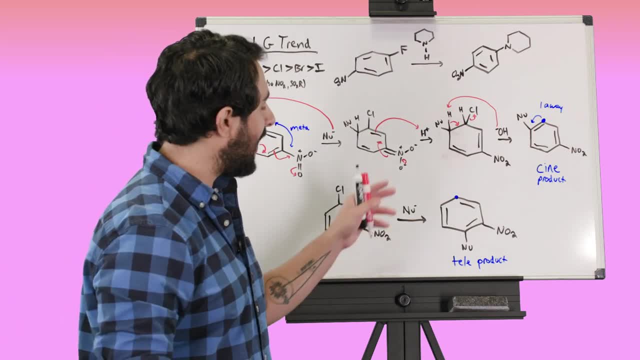 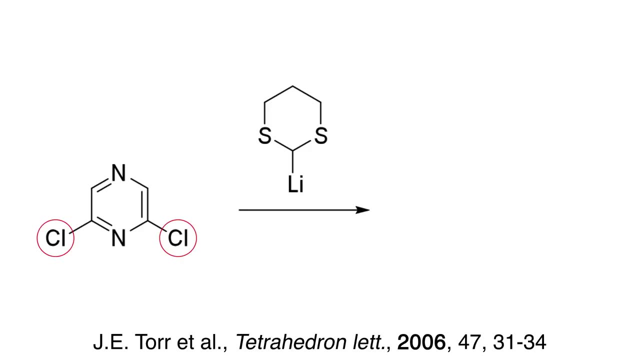 on that regiochemistry And so we actually see Sine and Tele substitution quite a lot in the literature. So a real-life example from the literature is shown here. The authors tried to replace one of the chloro groups in 2,6-dichloroperidazine with a dithiane. 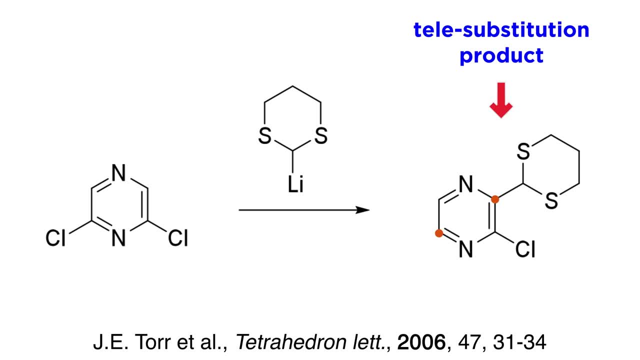 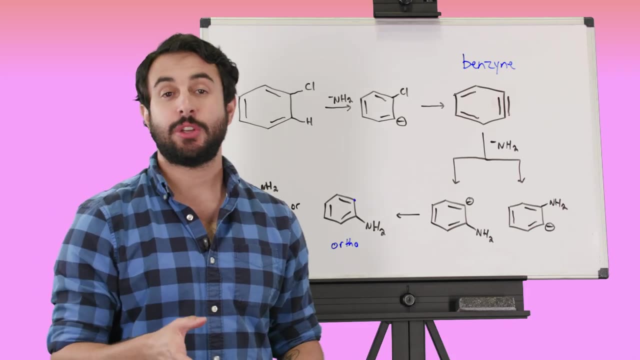 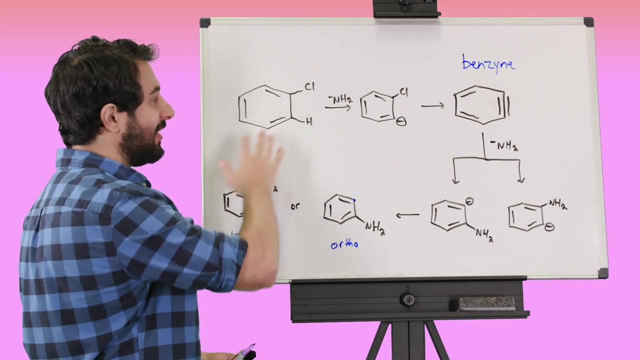 anion, But instead they got a Tele substitution product. Okay, And so we can see that these substitutions are pretty common in the literature, especially among heterocyclic compounds. So let's go over one other very important example. We can see that sometimes we can do nucleophilic aromatic substitution even when there is not. 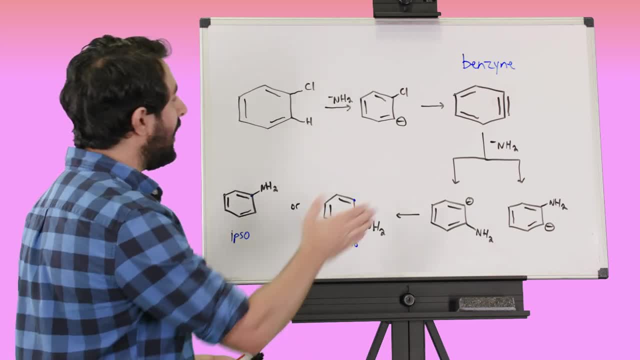 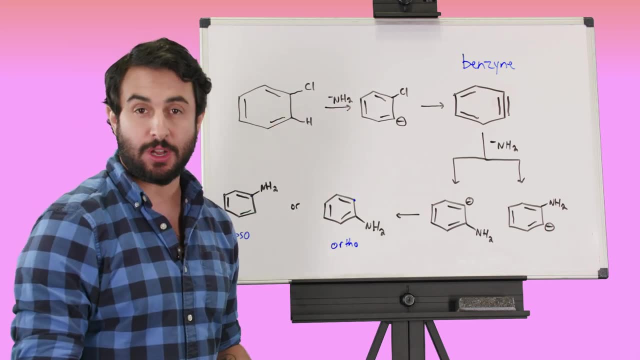 a special electron withdrawing group to stabilize the intermediate, and that can be done when we have extremely basic nucleophiles, So NH2-. we know that's a super-duper strong base. It's such a strong base that its conjugate acid, ammonia, is a base. 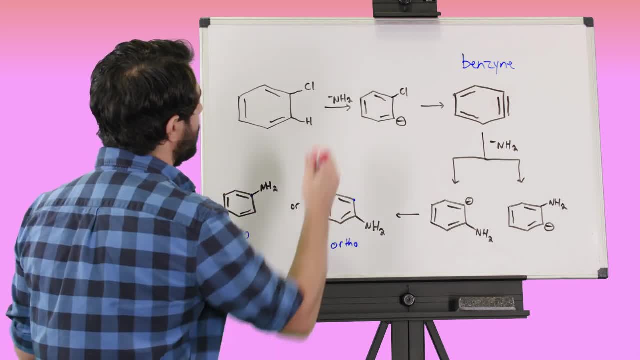 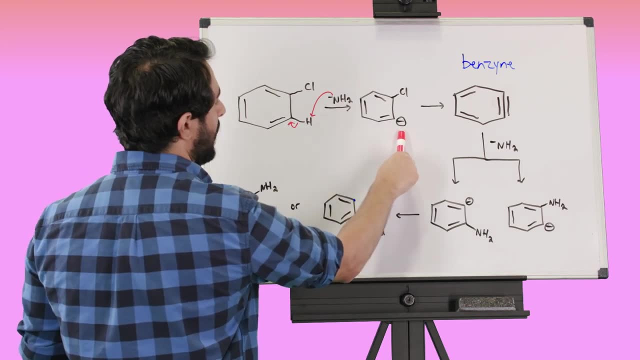 So super strong base, And what we see here is this is going to go ahead and grab a proton and that'll leave that there, And so we've got this intermediate. This is a little bit strange. We typically do not see this kind of a situation. 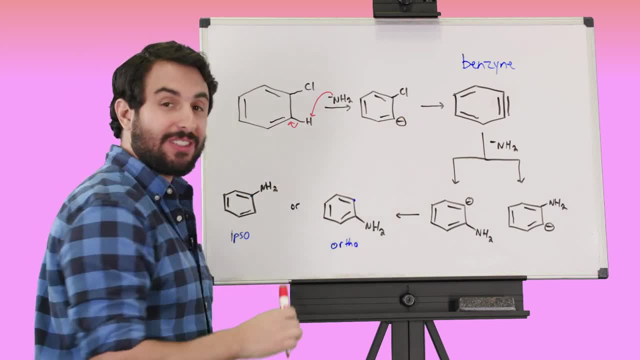 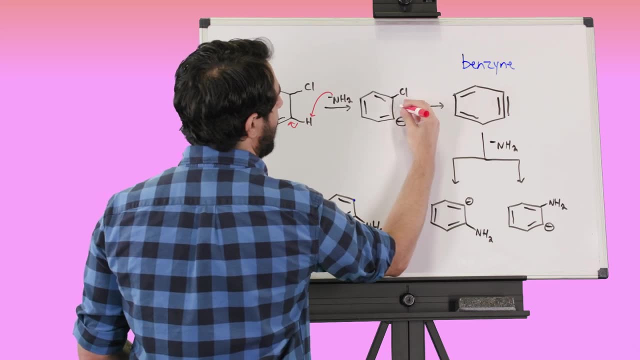 We have a formal negative charge on that benzene ring Again. that's just because this base is so exceptionally strong. Okay, So this is the rate-determining step. So this can go ahead and do this, pop off that leading group and this is going to produce. 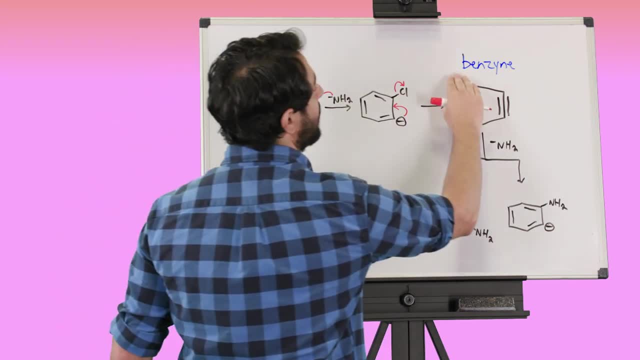 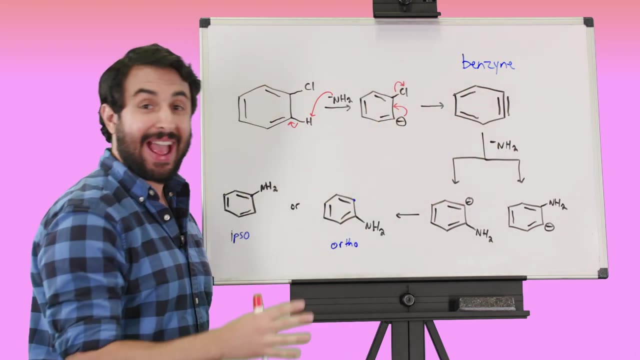 something that will seem extremely strange if you've never seen this before. This is called benzene, So that is a triple bond right there. So this is an extremely strained alkyne. We know that alkynes like to be linear. Those are sp-hybridized. 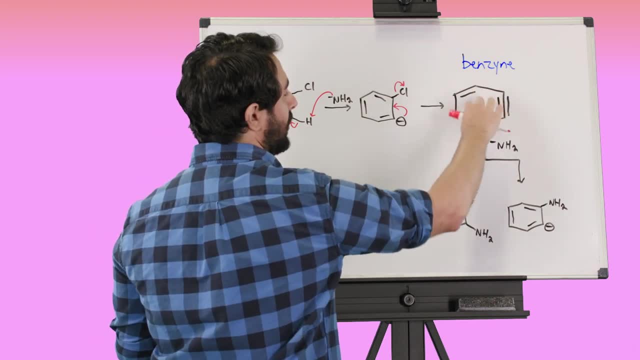 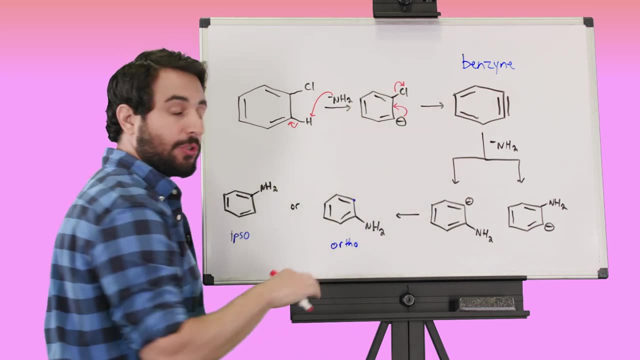 They want 180-degree bond angles. So to have to fit into this cyclic structure It's very strained And this is the rate-determining step. So for that reason this returns to the normal leaving group trend that we would expect. 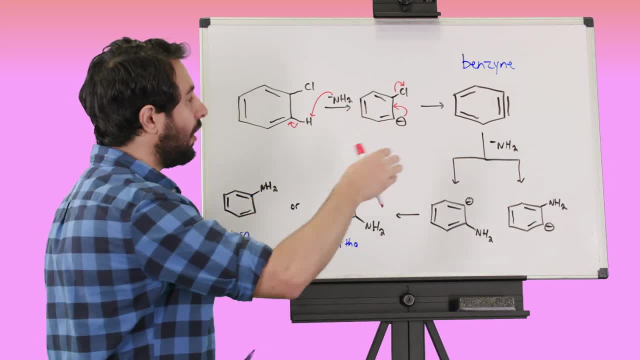 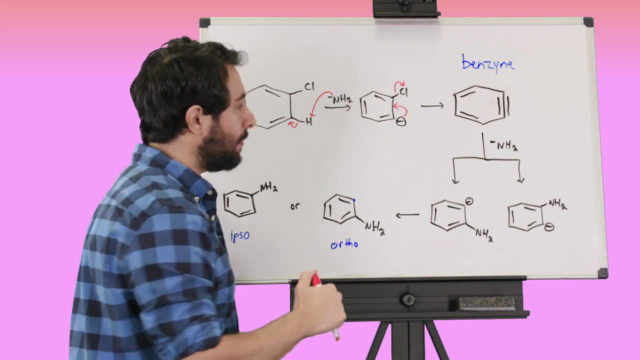 So the more stable the halide ion once it's left, the better the leaving group it was. So this is benzyne, Again. a little bit weird, but this is the intermediate that we're looking at, And we can use benzynes to do nucleophilic aromatic substitution, because now we still 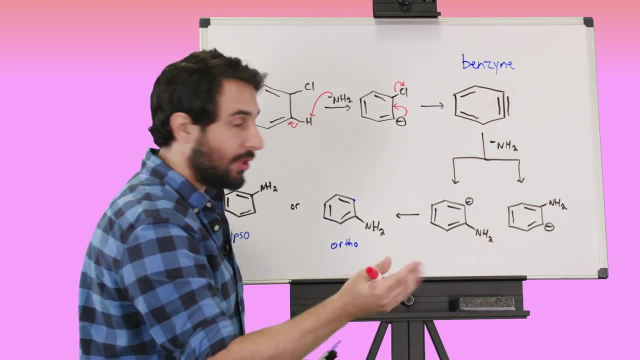 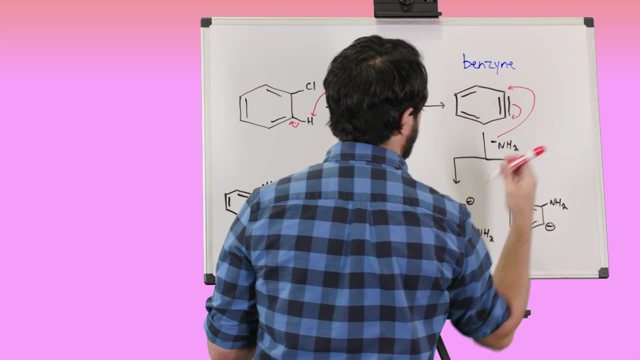 have some NH2- in there, can act as a base, can also act as a nucleophile, So this can go ahead and attack, Let's say this attacks right there and pops this pi bond up onto that carbon. We're going to get this guy right here. 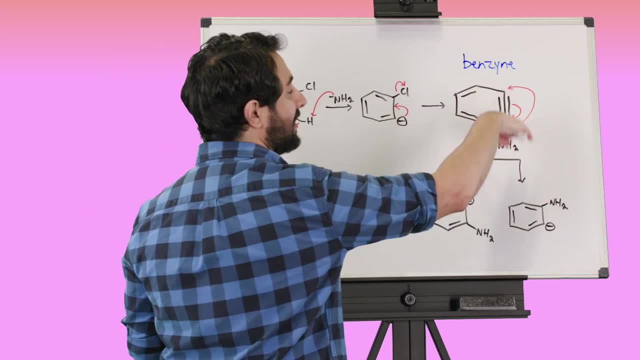 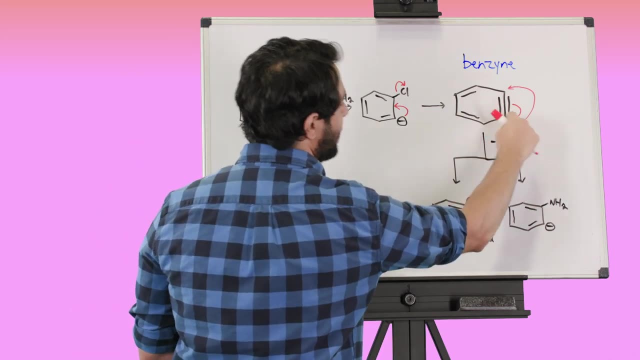 It can also attack at the other position, So this is totally symmetrical. The benzyne has lost any memory of where the leaving group was right, So this is completely symmetrical. This can just as well attack here and pop that pi bond up there. 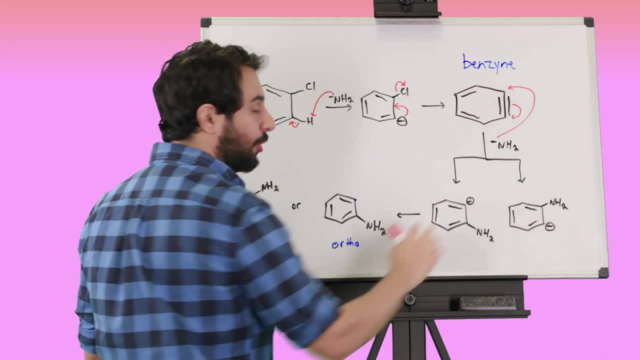 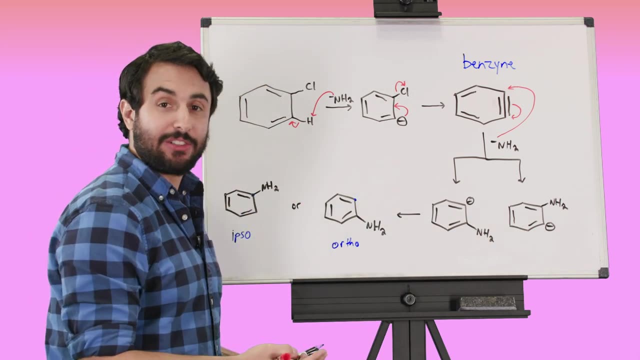 So we can also get this, And then from here these will just get protonated insolvent and we're going to get these two products And it is true that these are exactly the same molecule, but we want to be aware that. 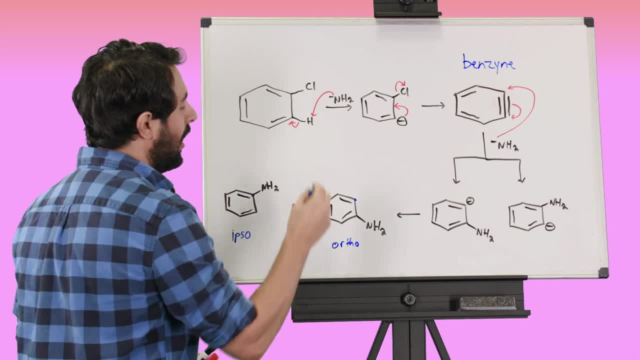 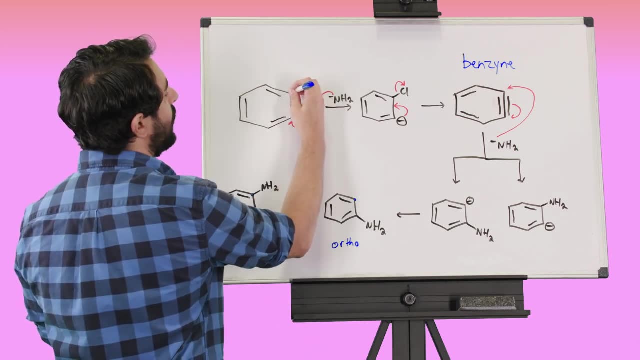 we would refer to them slightly differently if we had other substituents or something on there, The type of substitution that's going on, and we've discovered this through isotopic labeling studies. So if we labeled this carbon right here, so that even though the chlorine is gone- because 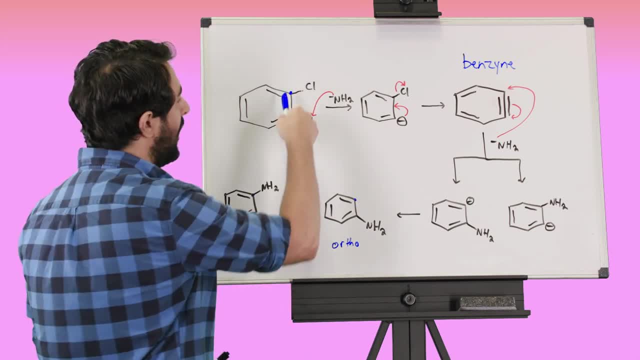 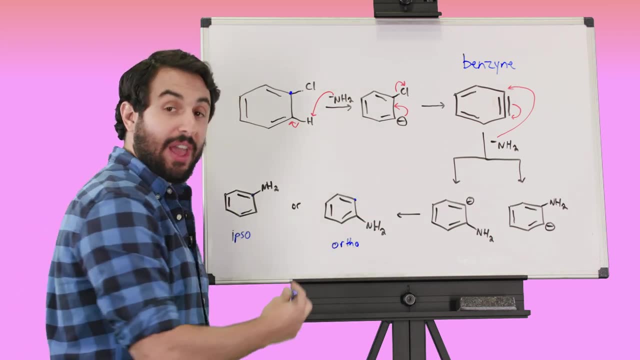 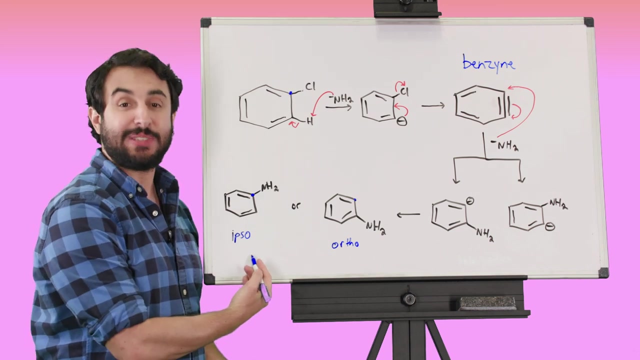 that's carbon-14, we would know which carbon it was and we know that if we have the incoming nucleophile next to this, Next to that carbon, we would call that orthosubstitution, And if we have that incoming nucleophile on the same carbon, we would call that ipsosubstitution. 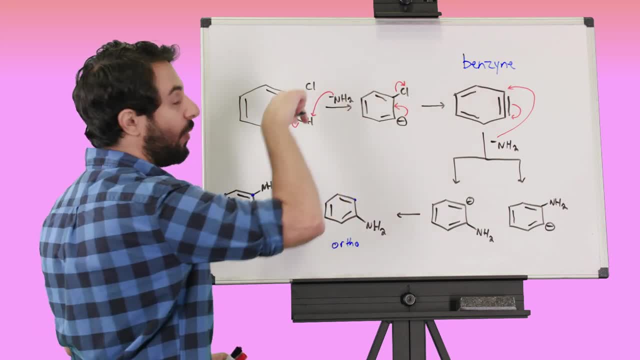 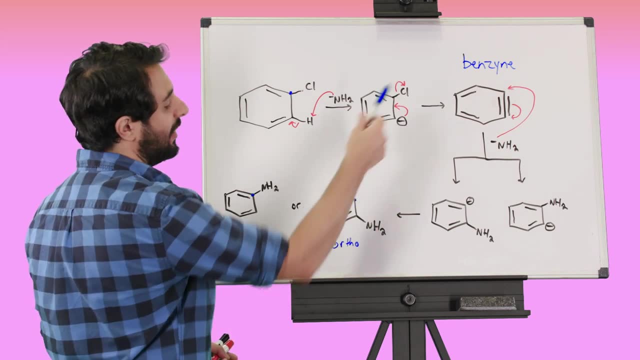 So, even though the benzyne has lost the memory of where the leaving group was, isotopic studies have told us this, and so this is important terminology, to know the difference, when using benzyne, between orthosubstitution and ipsosubstitution. 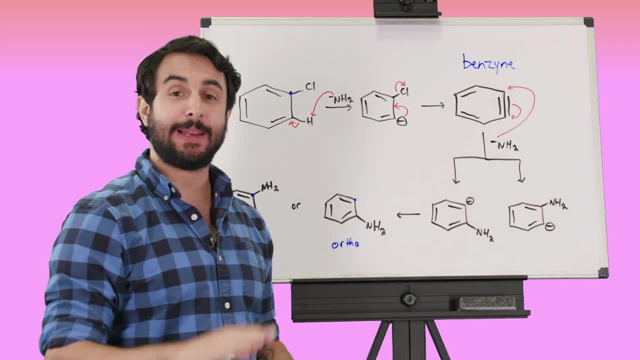 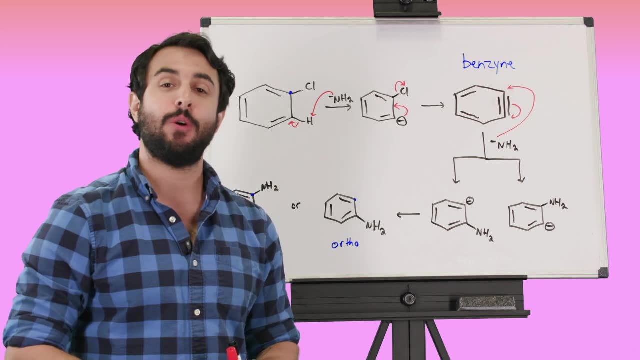 So we're going to talk a lot more about benzyne later. Okay, We're going to come back. This is a very important intermediate that we're going to look at some more later, but for now, hopefully that will help you understand a little bit about nucleophilic aromatic substitution. 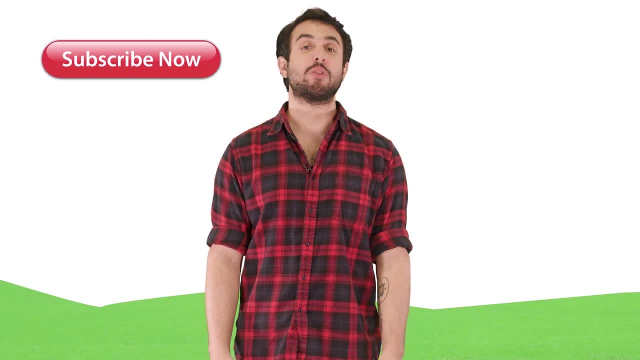 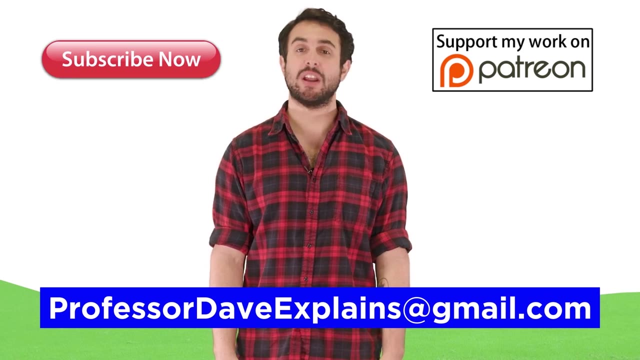 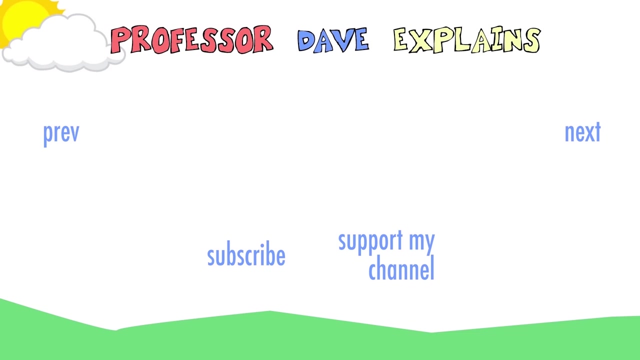 We'll come back for free today. Bye-bye, Bye-bye, Bye-bye, Bye-bye.